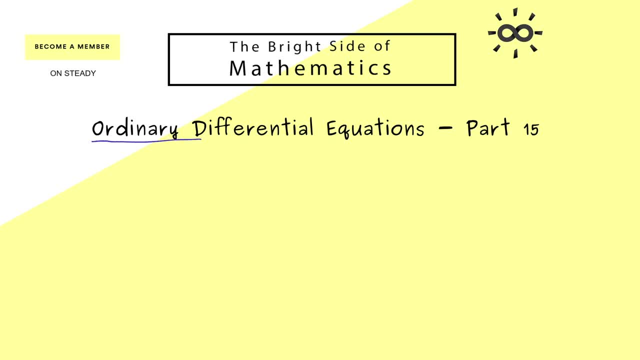 Hello and welcome back to ordinary differential equations, the video series where we discuss dynamical systems described by differential equations, And indeed today, in part 15, we will look at a more demonstrative way to visualize solutions of an initial value problem. More concretely, we will look at the so-called phase portrait and the orbits inside And let's 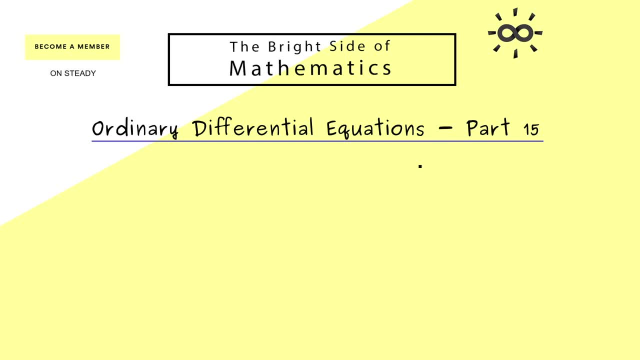 use what we have already learned to describe the orbits in a more mathematical way. But before we start with the details, i first want to thank all the nice people who support this channel on steady here on youtube or via patreon. I always say it, but i actually mean it, because you are the reason 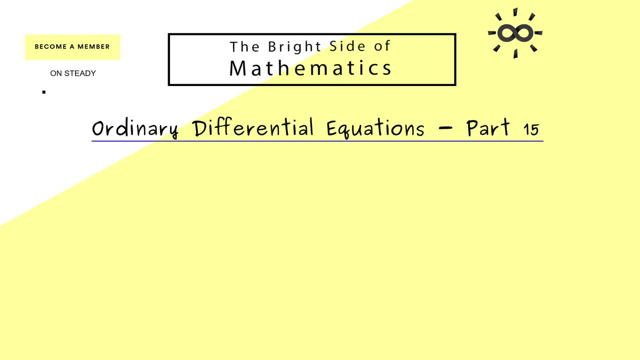 these videos exist and therefore you find the rewards for supporting me with the link in the description. Okay, then let's start with the topic, and you already know, we always look at systems of differential equations written in this first order here. This is not a restriction at all, as you already know, and v can be seen as a vector field. It maps rn into rn. 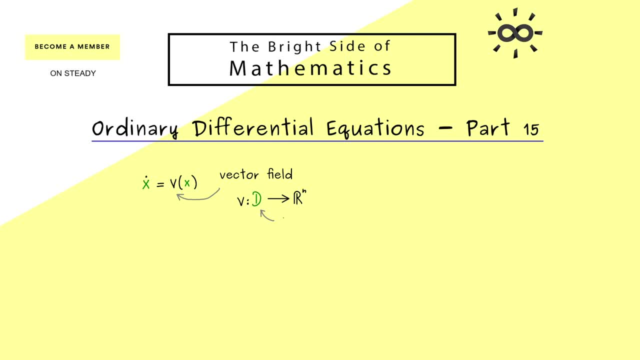 or, more generally, it's defined on an open subset in rn. And then, please recall, we can visualize that, for example here: if d lies in r2, we have this directional field. So at each point p in d, we put the vector v of p to it. Moreover, we also learned that an orbit is simply a curve inside. 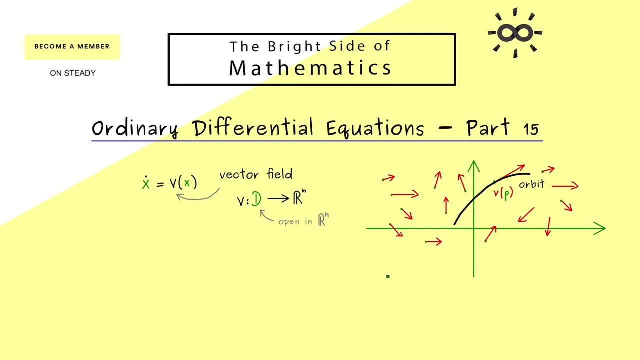 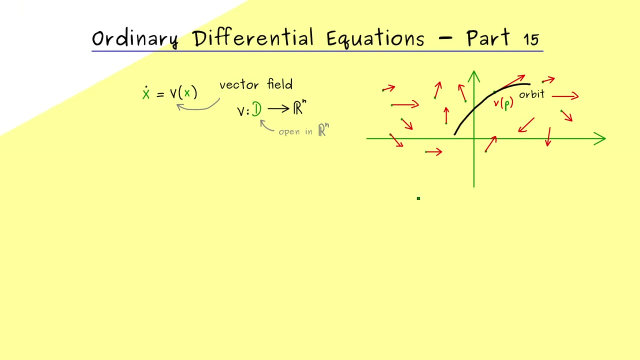 here that is tangent to our vectors. So in some sense it's the image of a solution for our ordinary differential equation here And now. since we have discussed solutions in a general sense before, we can now also apply this knowledge to orbits. The only restriction we want to put in 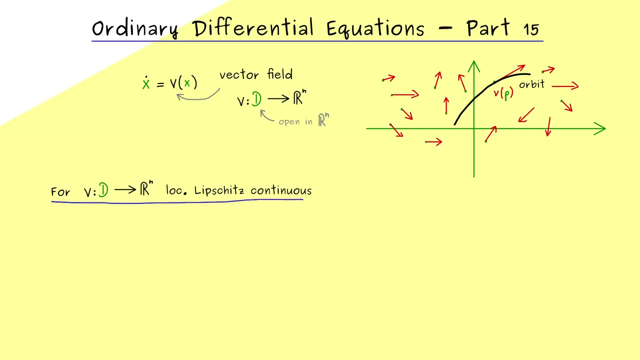 is that v is a vector And the V of p is a vector. Here is the vector where the vector v of p is. here is a locally Lipschitz continuous function, Because then we have our famous uniqueness and existence result for our initial value problem. And, as in the last video, in order to keep the 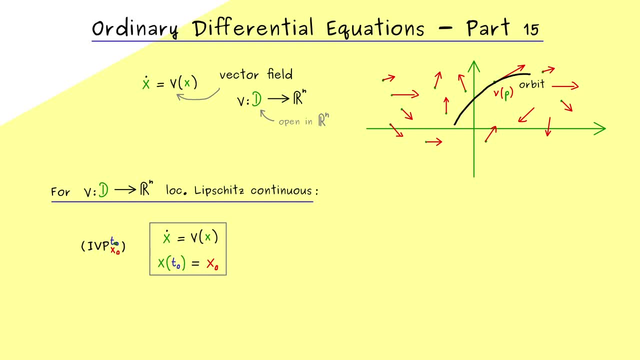 notation short: we will always write IVP with t0 and x0.. In addition, the last video has told us that this initial value problem has a unique maximal solution. So we also have the existence and uniqueness if we look at maximal solutions, Which simply means that the domain for the 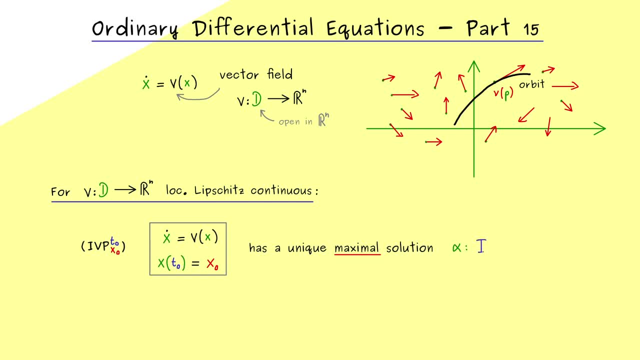 solution: alpha is given by an interval, i, and it cannot be made larger. So this is the best function we get as a solution for the initial value problem. However, of course we could change the time variable, which means we could translate the variable, So you could say a function beta of. 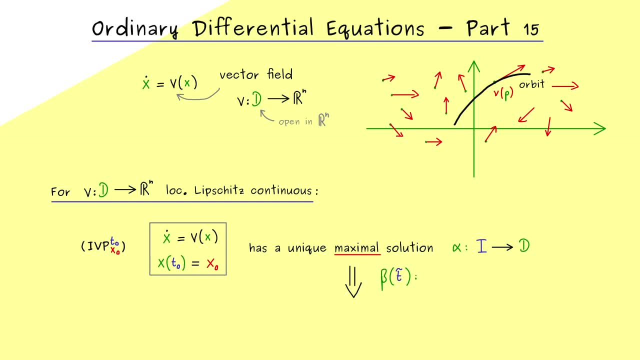 t tilde is defined by a function beta of t tilde By shifting the variable in alpha. So i mean we just have t tilde plus t0 inside alpha. Now, obviously this does not change the derivative at all. So the ordinary differential equation: 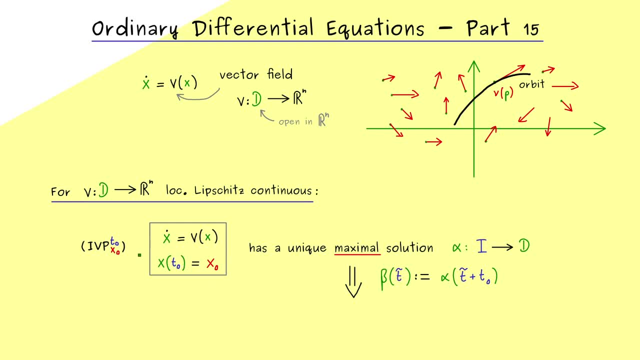 here is still satisfied, But it changes the initial value condition here In particular. you see, if you put in 0 into beta, then we get out x0 as well. Hence the function beta, where the interval i is also simply translated, is also a maximal solution of an initial value problem. 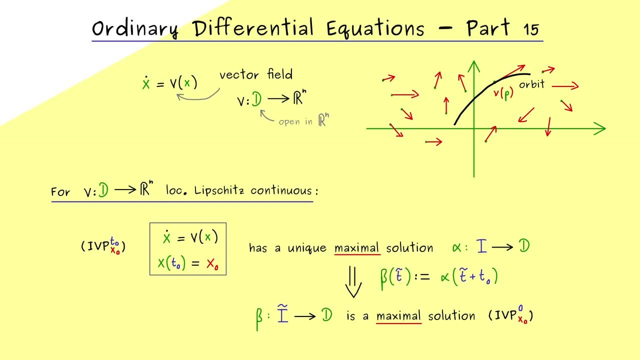 However, there the time starting point is set to 0. So in the end we see shifting the time variable like that is not a big deal. We just change the maximal solution in that way, Putting it differently: if we have the maximal solution for the time starting point 0, we have it for. 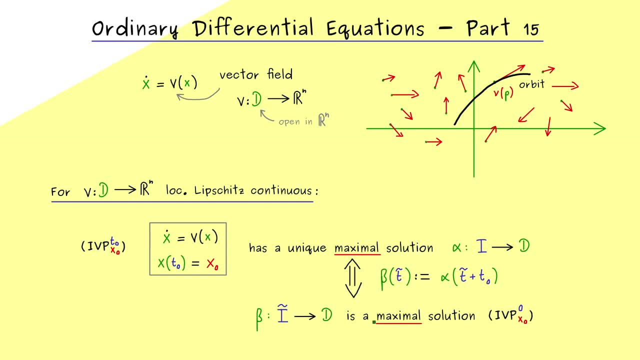 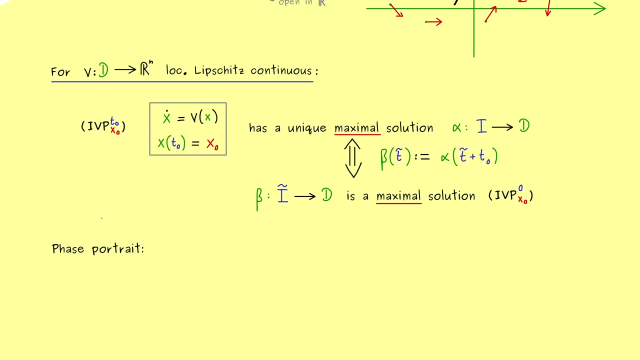 any other starting point as well know, because the orbit in this picture here does not represent the time variable anymore. therefore, it's important to know that this does not change our uniqueness result at all. okay then i would say, with this knowledge in hand, we can talk about the face portrait. 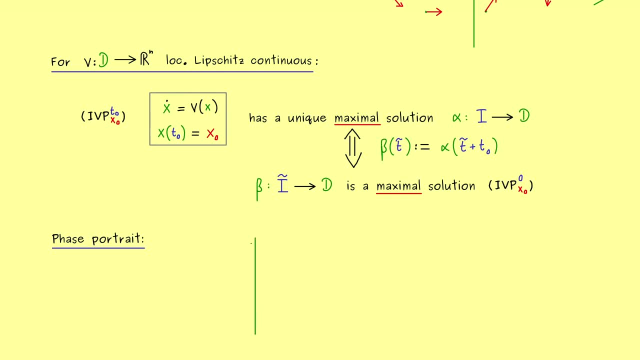 as a picture. it's not so complicated. it's again visualized in rn or more concretely, in our domain d, and now we can simply put all the orbits we have into this picture here and there. the question is: what are the restrictions for the orbits? indeed, we could think of a lot of funny orbits. 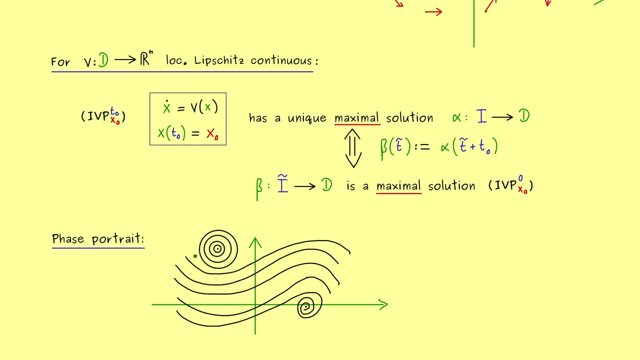 but the important question is: what is the mathematical definition of such an orbit? for example, we could ask: what is an orbit at a chosen point? x0 here, and, as you can see in the picture, it should be a subset of x0.. and indeed, it should be given by the values of a solution alpha. moreover, since we now know we can, 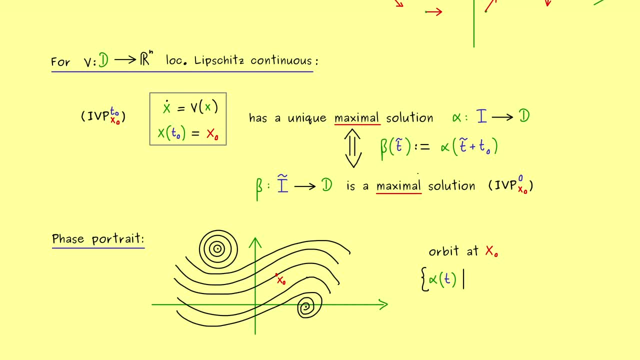 choose a maximal solution. alpha should be this maximal solution from before and then t just goes through all possible time points in i and i is just the domain of our maximal solution. alpha of the initial value problem. indeed, here it's important that we fix the initial value at x0. 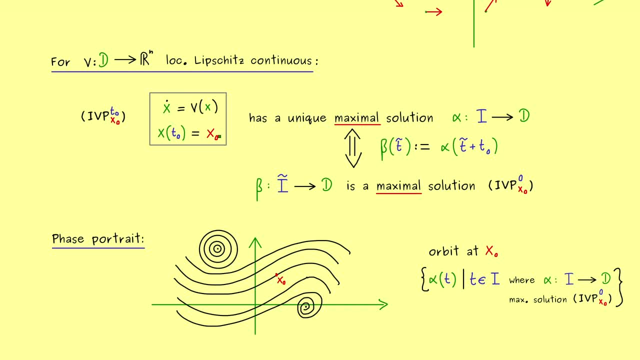 but the time value at x0 is not the same as the time value at x0 variable. the time starting point is not important, Simply because if we change it, we will change the solution function, but not the collection of the images of the solution function. In the end it. 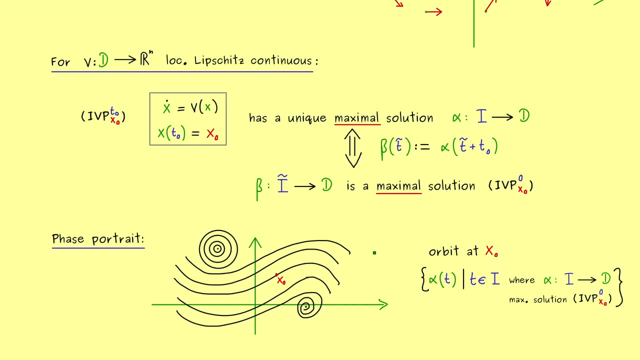 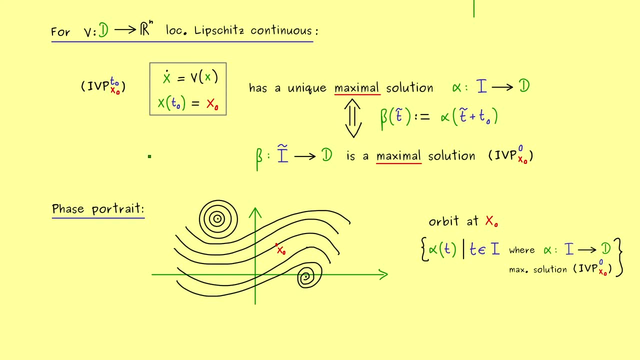 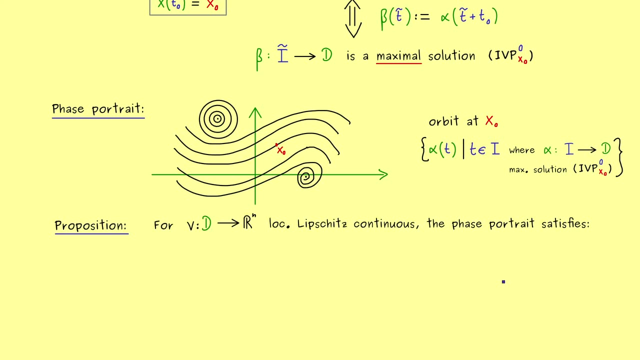 still hits the same points in Rn. Therefore, we have a very nice result of the phase portrait for a locally Lipschitz continuous function v, So let's formulate a whole proposition for this fact. Indeed, I could already summarize what comes now by saying that the orbits split up the whole. 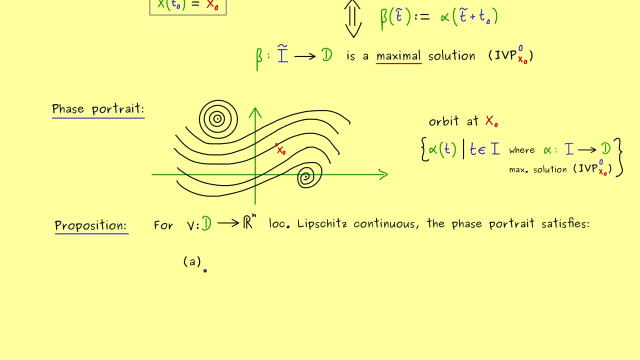 phase portrait, And by this we essentially mean two important points: existence and uniqueness. Maybe first the existence for all points in the domain D. we have an orbit, So we have the existence of such a set. we now just call O, And the idea here is that X lies on such an. 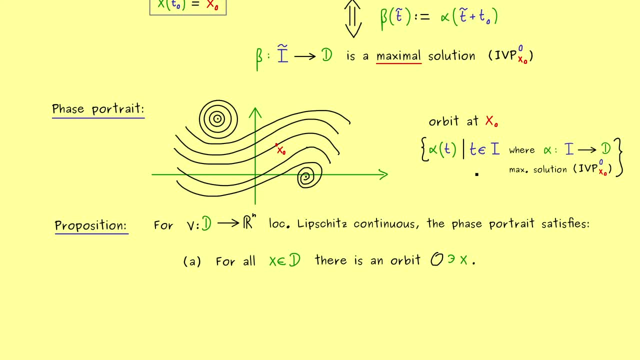 orbit. So we have the existence of such a set. we now just call O And the idea here is that X lies on such an orbit, And obviously this is what we get, because we have the existence of maximal solutions for the initial value problem, now starting with X. So this means there are no gaps in the phase portrait. Each 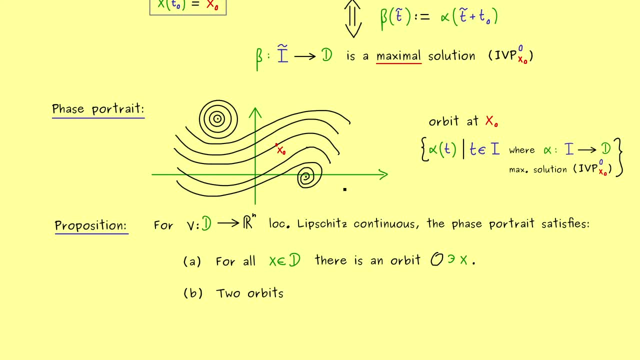 point has a corresponding orbit And we also already know each point can only have exactly one orbit. In other words, two orbits, O1 and O2, cannot cross. If it happens that they cross, which means they have a non-empty intersection, then the only possibility is that they were. 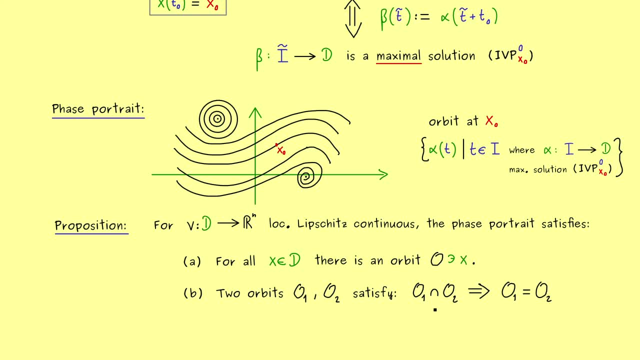 already the same. In fact, this is now easy to prove because you already know how to shift the variable in different orbits. So you see, the proof here is already done, simply because we know that in the definition of the orbit we can use the unique maximal solution. Therefore, I would say: 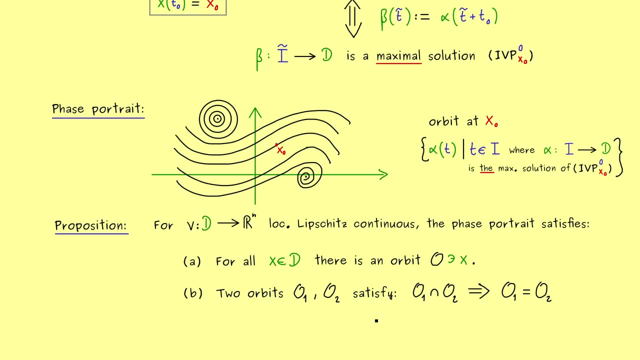 in the next video. we can apply this knowledge to examples and we can look at some special orbits. For example, this circular orbit here could be a periodic orbit, which means if you go through it with the time variable t, so you increase t, then you hit some points infinitely many times And a singular case of that would 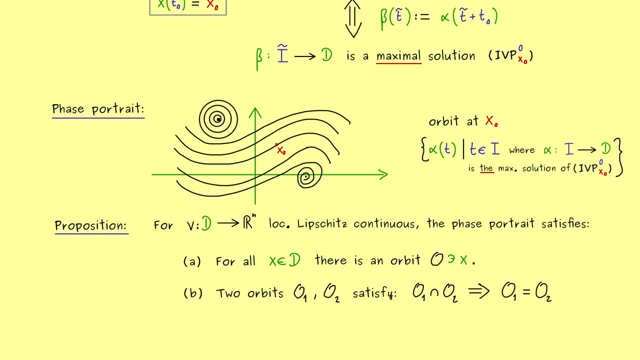 be the orbit here given by just a point, which obviously represents a constant solution And, speaking in dynamical terms, this would be a fixed point for the dynamic given by the ordinary differential equation. However, let's discuss that in the next video. So I hope I meet you again and have a nice day. Bye, bye. 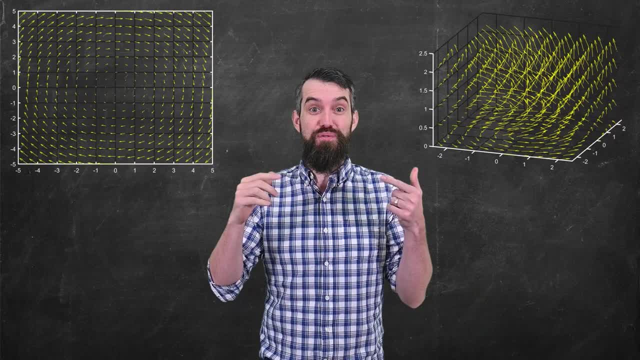 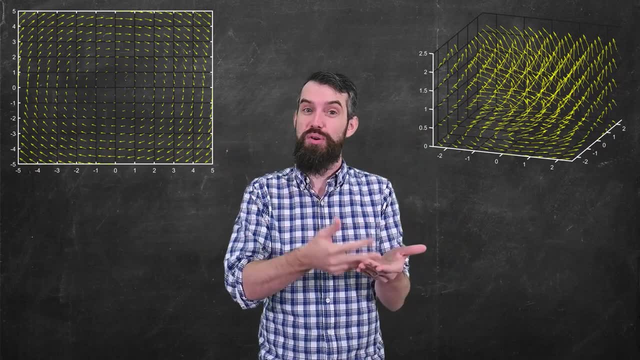 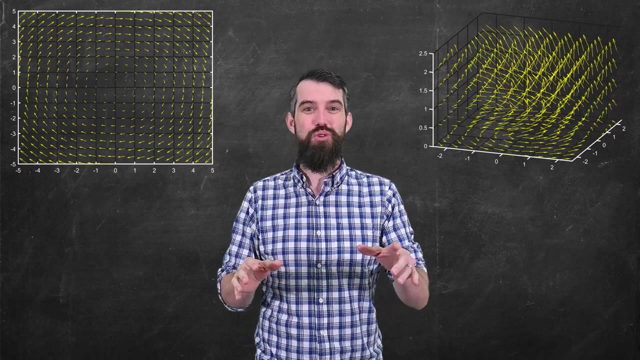 Welcome to Vector Calculus. In this video I'm going to give a bit of an overview of the big ideas, the big themes that we're going to see in Vector Calculus. And actually this video is the first video in an entire playlist on Vector Calculus. that corresponds to about the first third of my course as a professor at the University of Victoria.